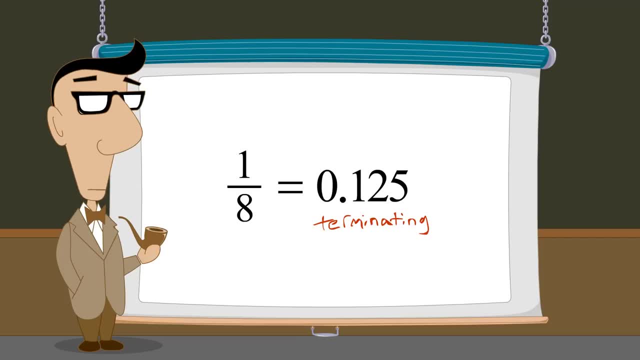 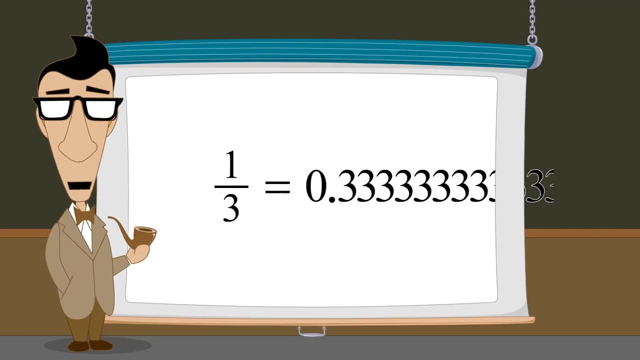 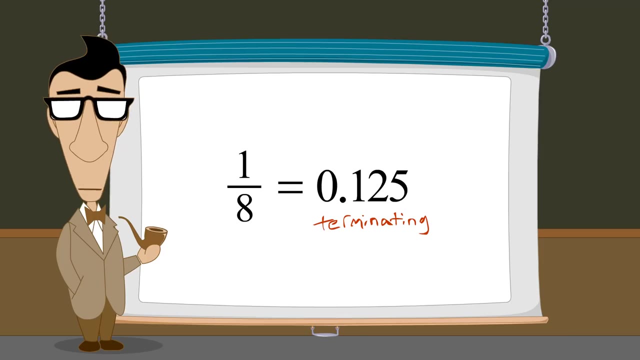 This decimal number will either terminate, meaning that it can be represented with a finite number of digits, or it will have one or more digits which repeat forever. In this lecture, we will see how to convert any terminating decimal number back into a fraction. Remember that each digit in a decimal number 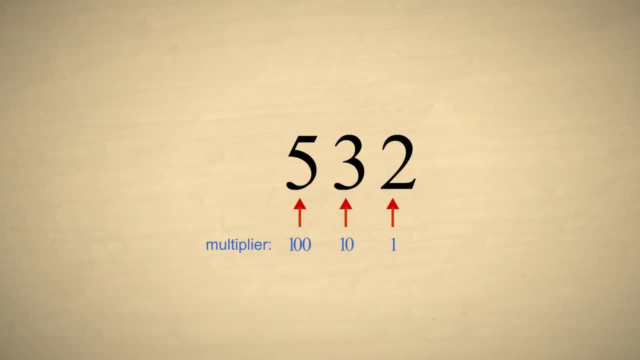 represents a value ten times that of the digit to its right. Now, if we take any decimal number and multiply it by ten, each digit is shifted one column to the left. We have increased the value of each digit by a factor of ten. This is also true when there are digits to the right of the decimal point. 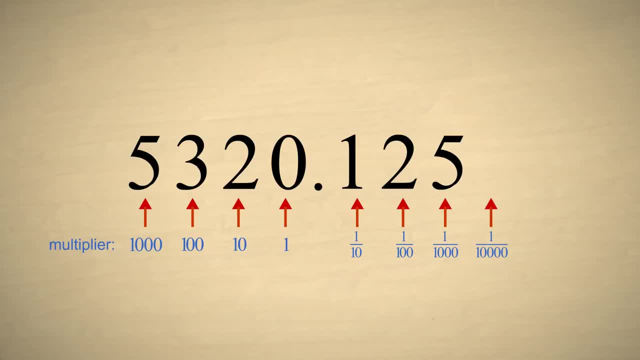 For example, the decimal equivalent to the fraction one-eighth is 0.125.. If we multiply this number by ten, each digit is shifted one column to the left. If we multiply by ten, again, each digit is shifted one more column to the left. 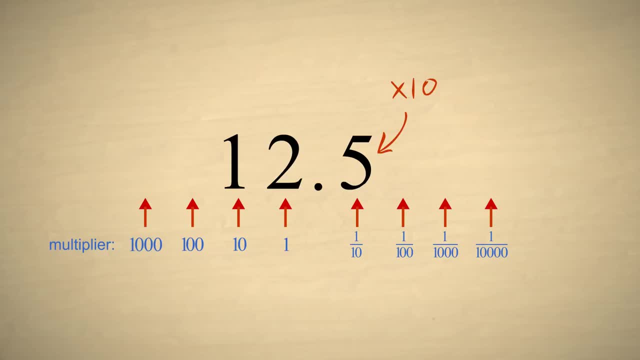 And if we multiply by ten a third time, there will be no more digits to the right of the decimal point. We will have an integer. So by multiplying our decimal number by ten three times, which is the same as multiplying by one thousand, we have produced an integer. 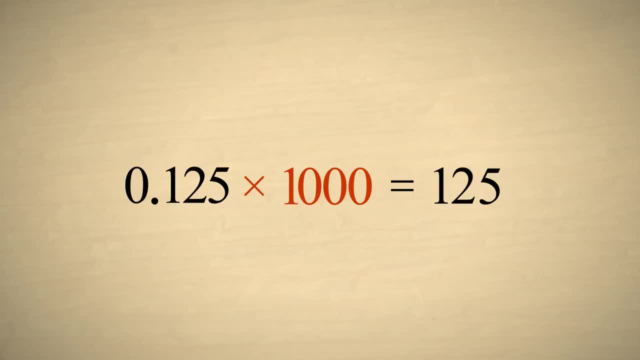 which is one thousand times the original number. If we then divide the integer by one thousand, the result will be equal to the original number. So 0.125 is equivalent to the fraction 125- one-thousandths. Now, using the techniques we learned in our lecture on reducing fractions, 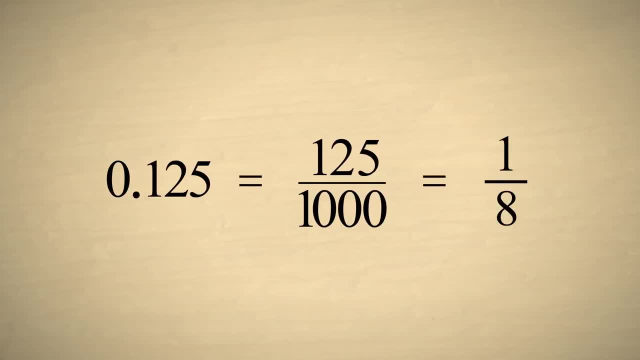 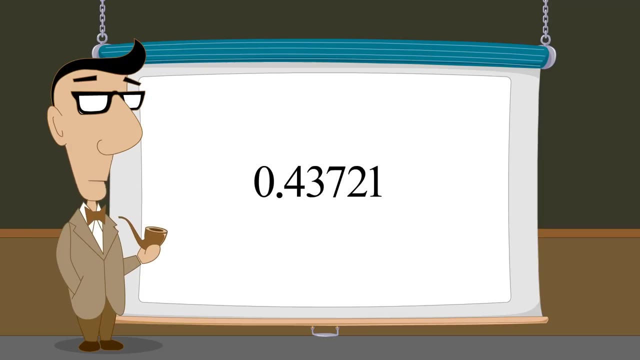 we can simplify this fraction to one-eighth. So we have converted the decimal number 0.125 to the fraction one-eighth. We can use this same technique to convert any decimal number with a finite number of digits to a fraction by multiplying it by ten, enough times to produce an integer.